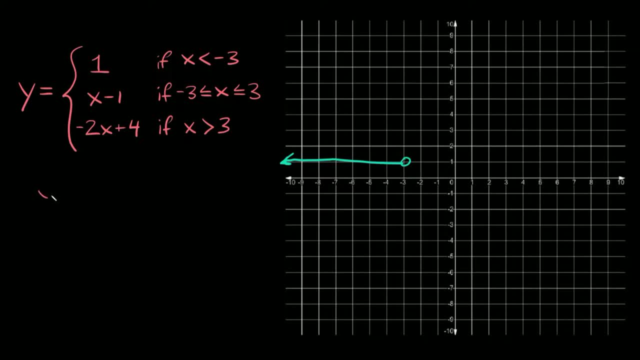 Okay, the next equation that we're going to graph is: y is equal to x minus 1, right, y is equal to x minus 1.. Now to graph a line, all you need to do is graph two points, okay, So we can make a. 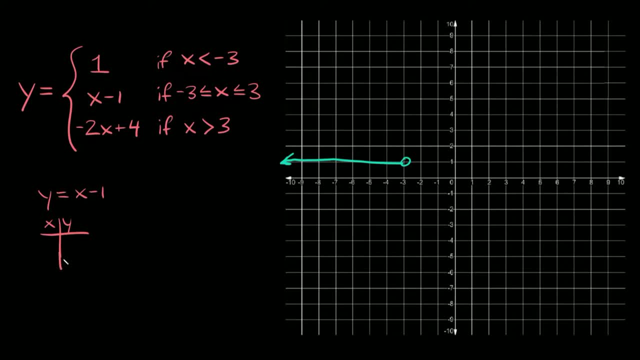 little xy table and just plug in two points here for x and see what pops out for y. Now what should we plug in for x? Well, for this equation y is equal to x minus 1, it's valid from negative 3 to positive 3, right? 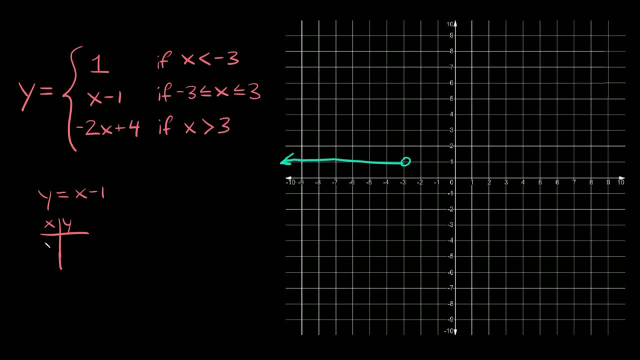 So those are the two numbers you're going to want to use in this case. So we're going to plug in a negative 3 and a positive 3.. Okay, so if we plug in a negative 3 into this equation, right here, 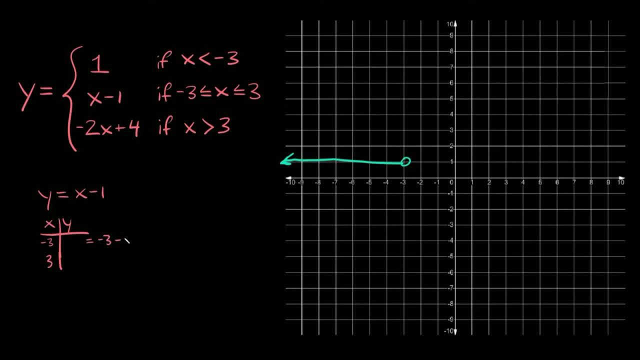 we're going to get that y is equal to negative 3 minus 1,, which is equal to negative 4.. And for this one it's going to be: y is equal to 3 minus 1,, which is equal to positive 2,. okay, So for this, 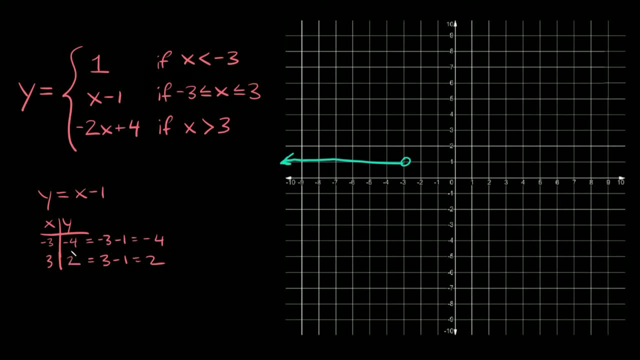 first one it's negative 3, and for the last one it's positive 3.. So we're going to plug in a 4, the second one is 2. so then these are the two coordinates that we're going to graph: negative 3, negative 4 and 3 comma 2. so first of all, negative 3, negative 4. 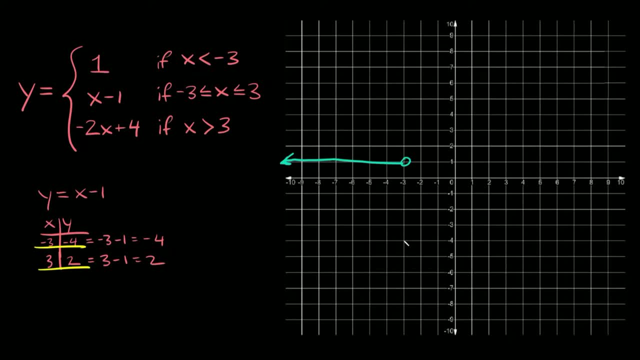 so negative 3, negative 3. negative 4 is right here. and is this going to be an open or closed circle? it's going to be closed right, because here we have a less than or equal to, and here we also have a less than or equal to, right. so both of. 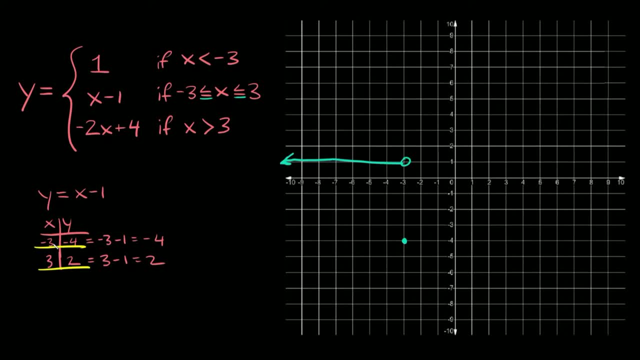 these are going to be closed circles, okay. so the first spot is at negative 3, negative 4, and the next one is that 3, 2 right, 3, 2 right there, okay, and then we're just going to connect the dots like that. okay, and I'm not going to go. 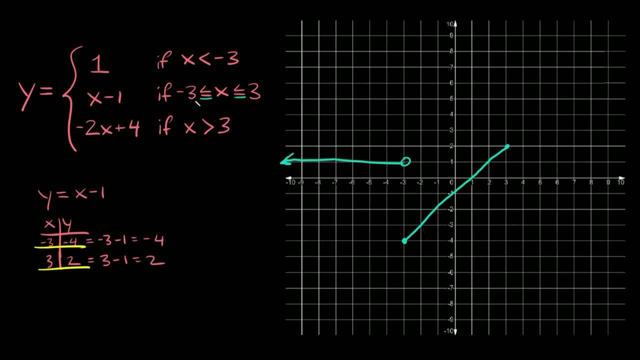 any further. right, because again, the limits for y is equal to x minus 1, goes from negative 3 to positive 3, right, so this is negative 3 and this is positive 3, so it's only valid for this space, right here. okay, now, lastly, we're going to graph. y is equal to negative 2x plus 4, so y is 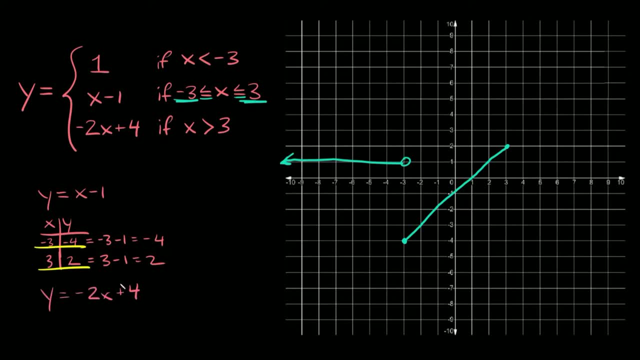 equal to negative 2x plus 4. okay, now this one is valid for wherever x is bigger than 3. okay, so if we make another little x y table right here, right, what numbers should we plug in? well, all our x values have to be bigger than 3, so we can plug in 3 and something bigger than 3 like 4. right, those are kind of 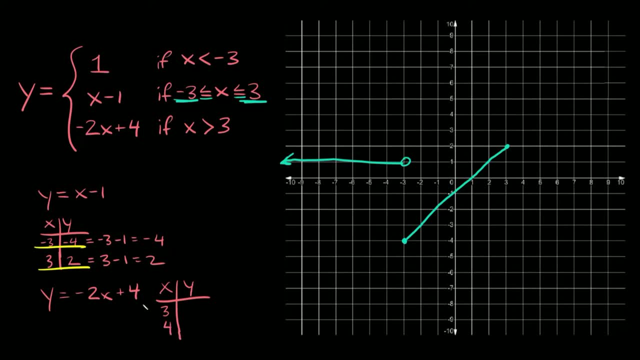 easier numbers we can work with here, okay. so if we plug in these two numbers into our equation right here, we're going to get that y is equal to negative 2 times 3 plus 4, and for this one it's going to be negative 2 times 4 plus 4. okay, so for this first one, negative 2 times 3 is equal to. 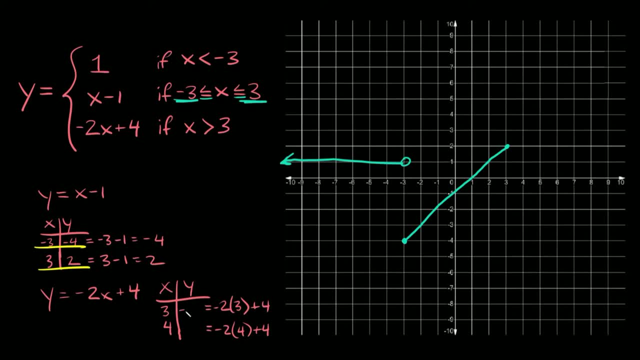 negative 6, and negative 6 plus 4 is equal to negative 2, and for the second one, negative 2 times 4 is equal to negative 8, and then negative 8 plus 4 is equal to negative 4. okay, so here are. 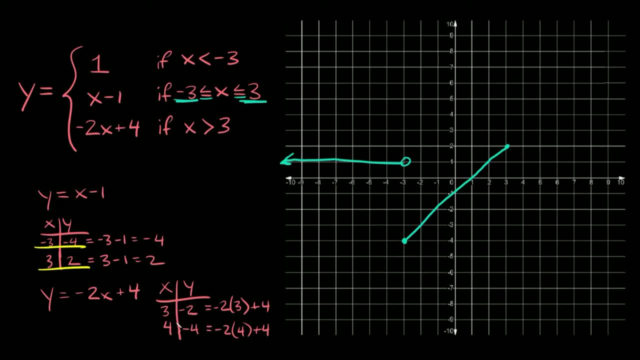 the two points we can plot for this equation: right here, so at 3 negative 2, and 4 negative 4. right, so 3 negative 2, right here. and are we going to have a closed circle or open circle? open circle: right, because our symbol over here is just a greater. 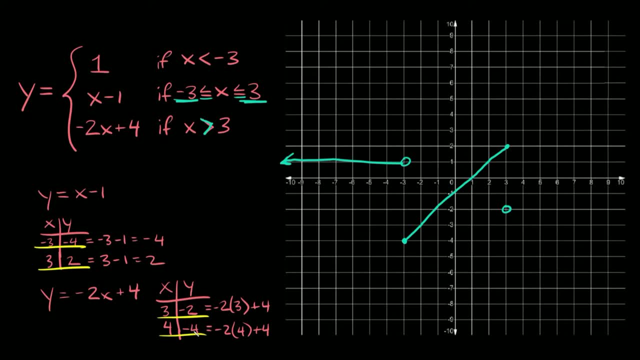 than symbol. and then our other point is at 4 negative 4. right, so 4 negative 4 is right there, okay. so then we're just going to draw a straight line like that and it just goes in that direction forever, okay. now, one thing i want to point out is that if we're going to draw a straight line, 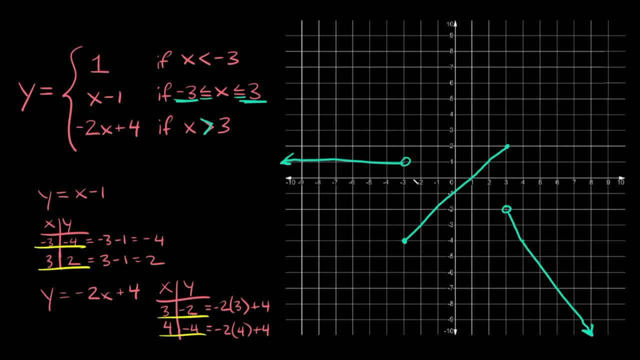 out here with the graphs is that they should never overlap. they should always line up exactly and vertically okay. so if i drew a line right here, you can see that both of the graphs line up exactly at the same spot, right at negative 3. right here they don't overlap right, this one doesn't come. 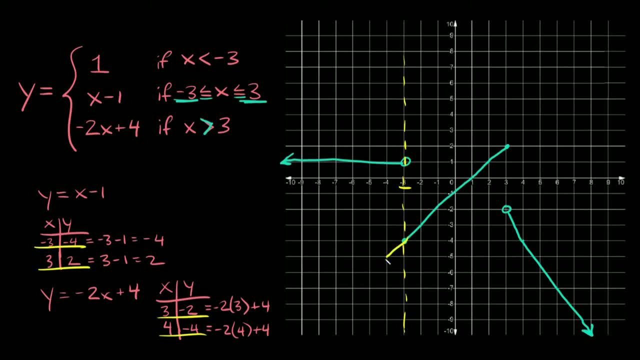 like over here, right, and this one doesn't come like down here, right? they don't overlap like that, they just line up exactly and it's the same thing with this other one, right? these should always line up exactly like that. so we're going to draw a straight line and then we're going to draw a.